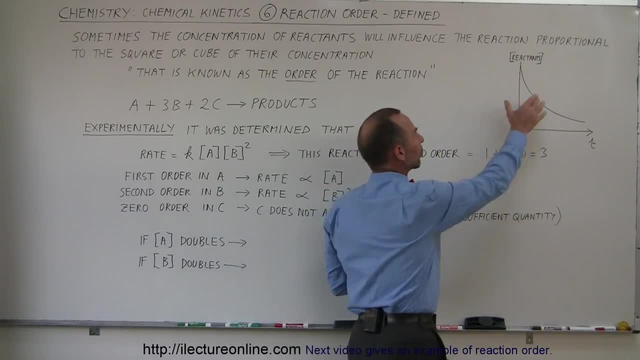 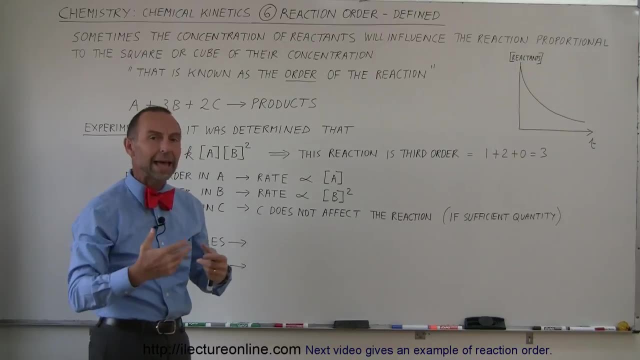 will be will be proportional to the concentration of the reactants. So the more reactants you have in solution, the faster the reaction will take place, and as the reactants are being consumed, the reaction will slow down. But then we realize that there's a dependency on the concentration of the reaction. Sometimes 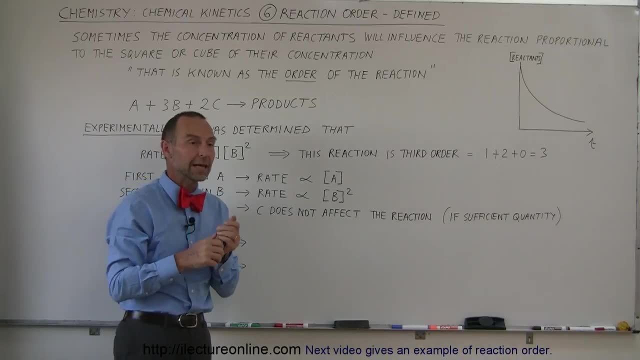 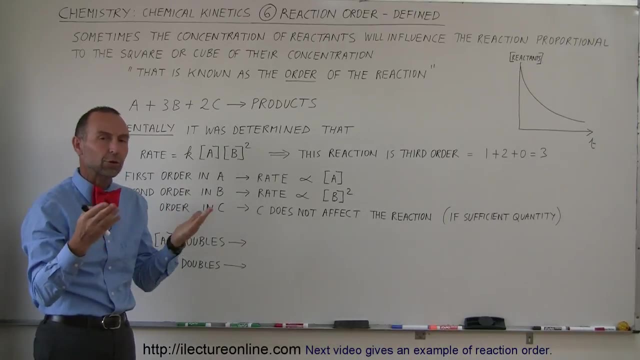 that dependency is not linear. Sometimes that dependency is in the order of the square of the concentration of the reactions or the cube of the concentration of reactions. So that's where the term order of the reaction or reaction order comes from. So let's read the definition here. It says sometimes: 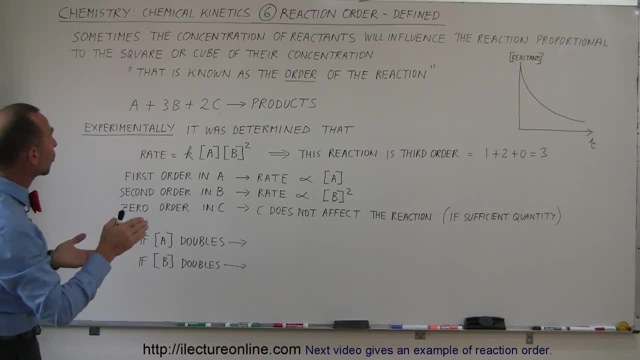 the concentration of reactants will influence the reaction proportional to the square or the cube of their concentration. Sometimes it's even to the concentration, to the 1.5 power or 2.4 power. Sometimes it's not even like the square or the cube. 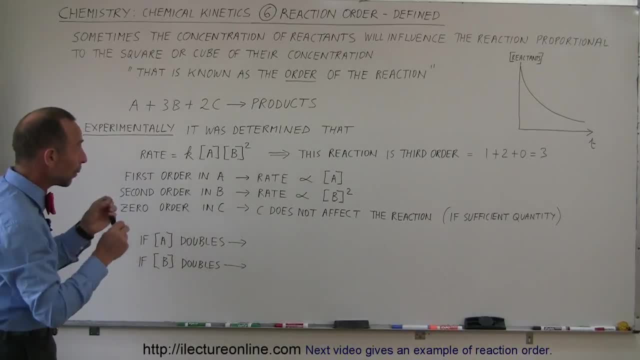 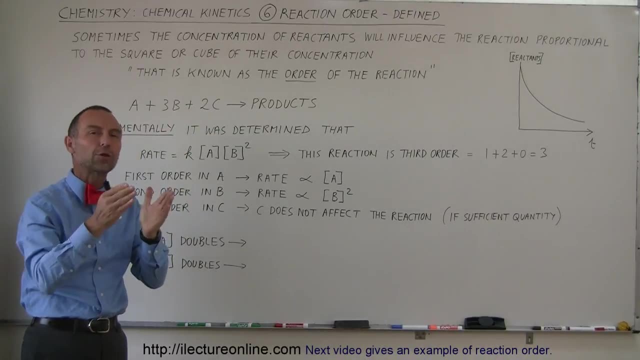 It can even be something other than an integer number, But whatever that is, that is known as the order of the reaction And of course, if there's more than one reactant, we have to add the orders together, one for each reactant. 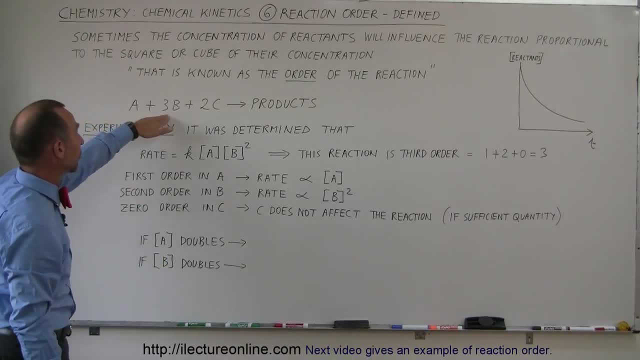 So for example, let's say we have the reaction A plus 3B plus 2C produces some products. Now A, B and C are some sort of molecule or some sort of atom. One, three and two- I didn't write the one here, but the coefficients here, of course. 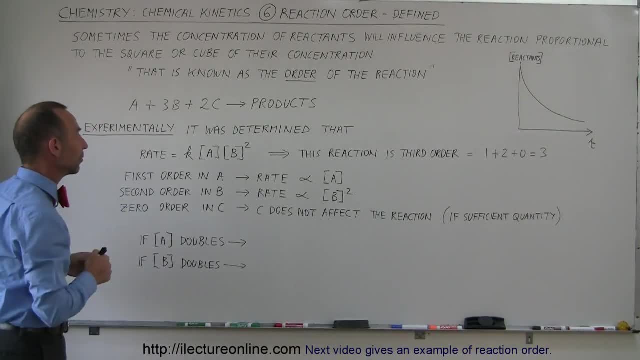 represent the number of moles you have to have in relation to everything else. Now it turns out that the order is not related to these coefficients in front of the reactants, For example. the coefficients simply represent how many moles you need of each reactant. 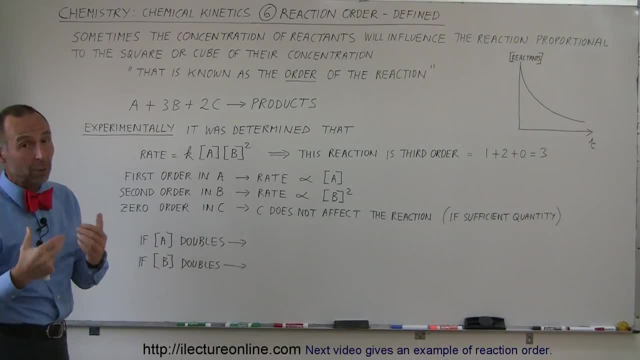 how many atoms you need, And that's not necessarily- and quite often not remotely- related to the order. So how do we determine the orders? Well, most of the time it's done experimentally, And in some future videos I will show you how we do that. 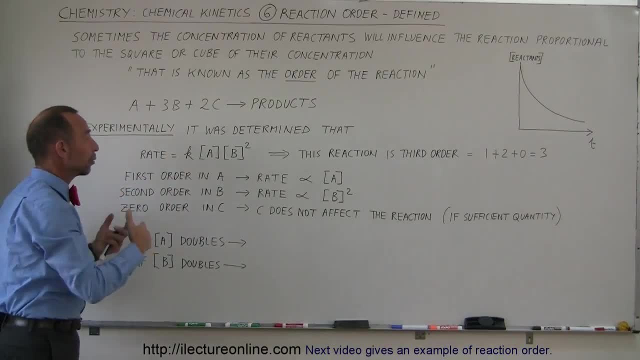 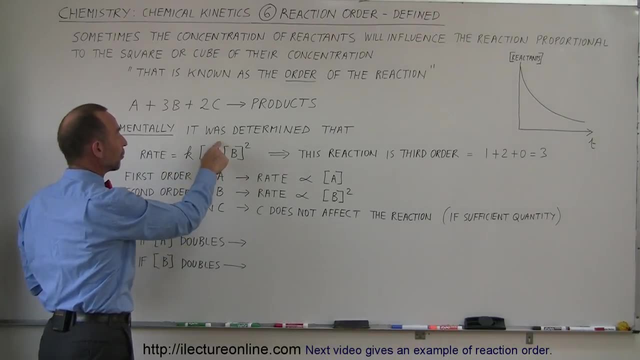 But right now let's say that we experimentally determined that the order of this reaction was that the rate is proportional to the concentration of A to the first power, the concentration of B to the second power, and it's not related, It's not dependent on the concentration of C. 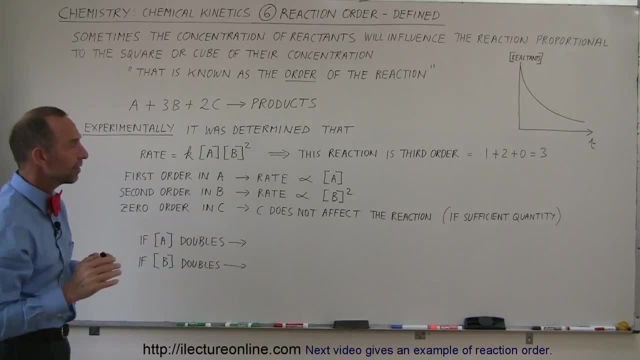 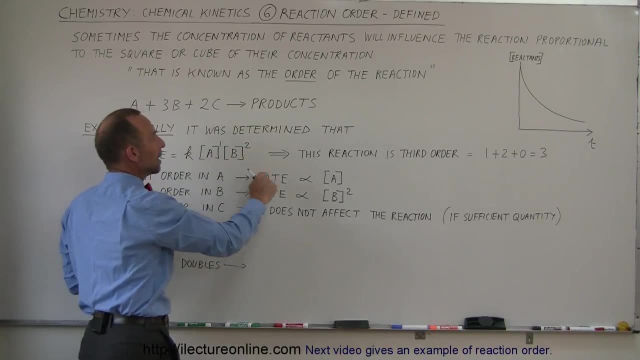 So that's why we don't have the C there. So therefore, we can say that this reaction is the third order, because we have the one for the concentration of A, we have two for the concentration of B and we have zero for the concentration of C. 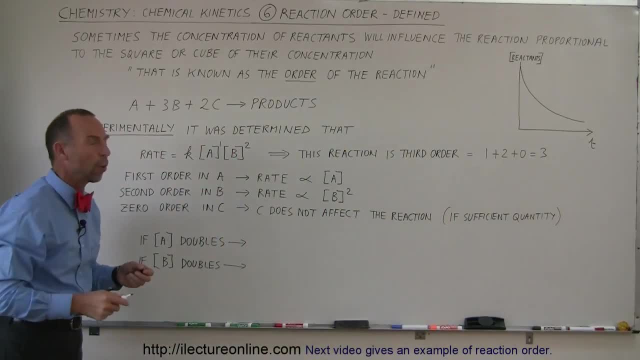 So one plus two plus zero gives us three, So it's the order three. Now, what does that really mean? Well, since we have a first order in A, that means that the rate is directly proportional to A. which other? In other words, if you double A? 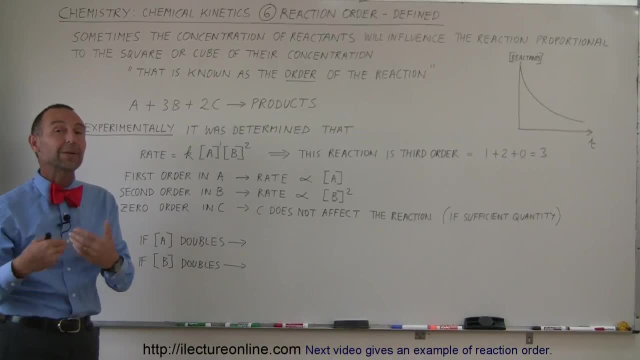 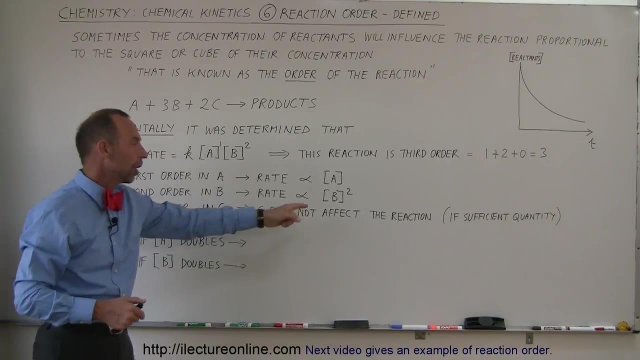 then you'll have twice the rate of the reaction. If you triple A, you'll have three times the rate of the reaction. Also, here we have B being the second order in B. That means if you double the concentration of B the reaction will be four times as fast. 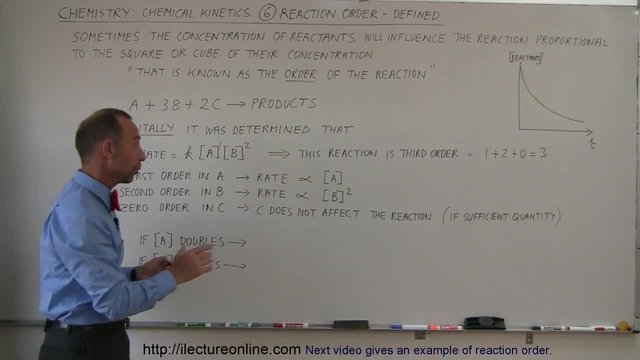 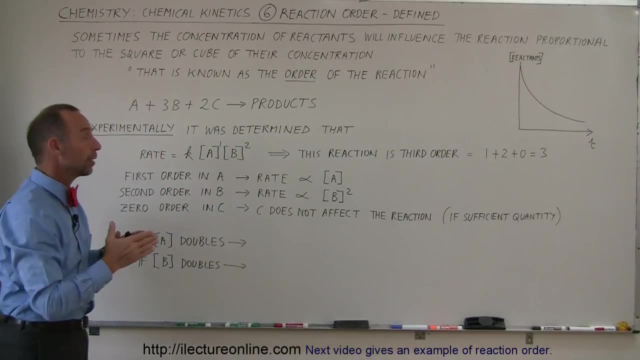 If you triple the concentration of B, it'll be nine times as fast, and so forth. In other words, the rate of the reaction is proportional to the concentration of B squared. And of course, since they're both there, we then say that the order of this reaction. 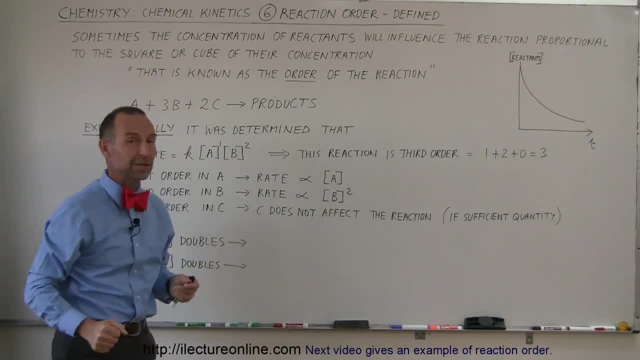 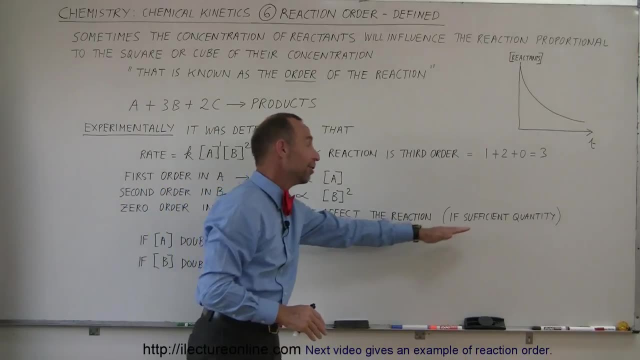 is one plus two zero for C, a total of three for this particular reaction. Zero order simply means C does not affect the reaction, as long as, of course, you have enough quantity of C not to inhibit the reaction to take place, because once you run out of C, of course. 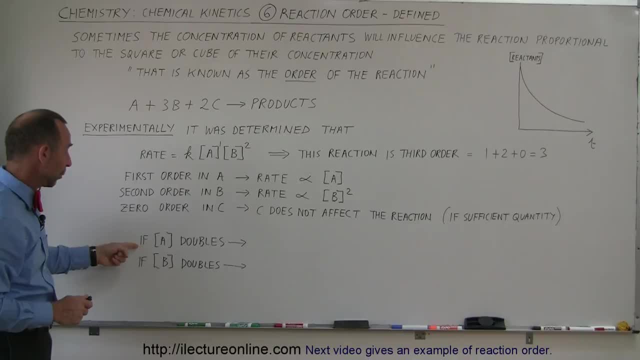 then the reaction will not continue. So again, what do we say then? If A or if the concentration- the brackets here simply mean if the concentration of A doubles, and if it's an aqueous solution, of course, then we're talking about moles per liter. 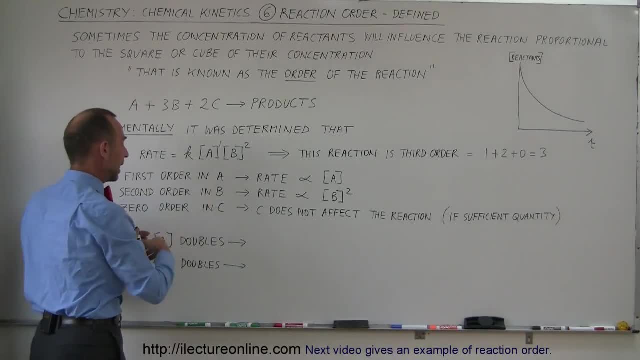 If the concentration of A doubles, what happens? Well, since it's a first order in A, that means that the reaction rate doubles. And now again quick quiz: What if the concentration of B doubles? Well, since it's a second order of B. 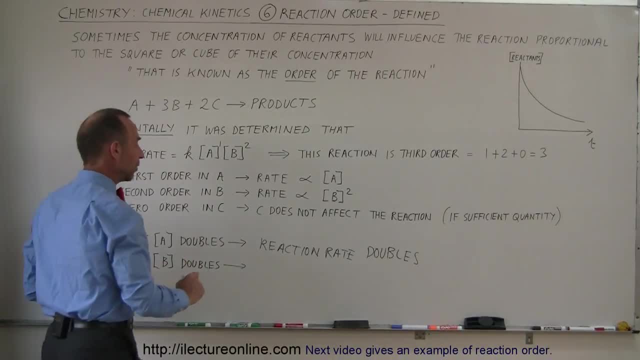 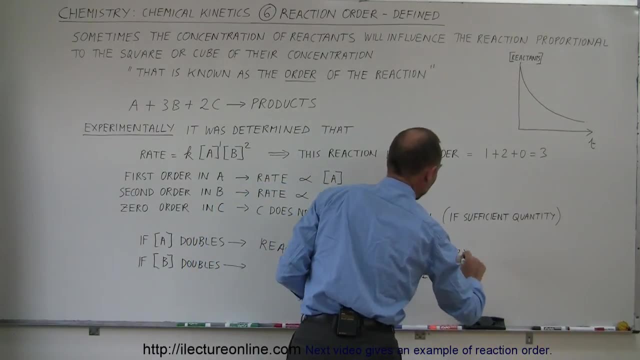 that means if B doubles, we'll have four times the rate, so the reaction rate quadruples. So it'll be four times as fast. only two times as fast for A. So if, if the concentration of A doubles, the reaction is twice as fast. 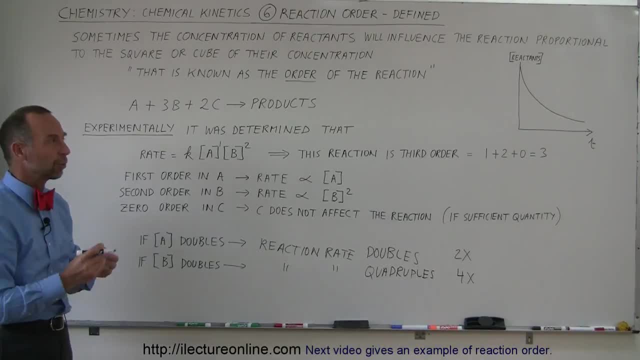 If the concentration of B doubles, then the reaction will be four times as fast. So that's what we mean by the order. And yes, we have to figure out what those orders are experimentally. You cannot simply look at the equation and say: